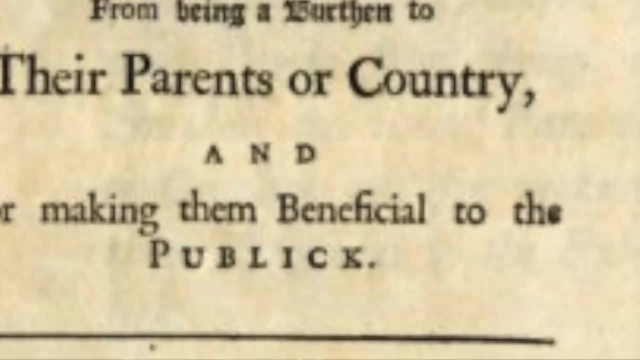 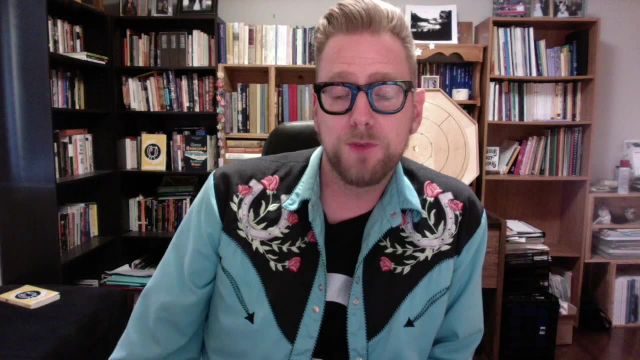 time and, of course, the author of books such as Gulliver's Travels. And in no way was he actually advocating that people take up cannibalism. In fact, the point of the pamphlet was to say the exact opposite. Saying the opposite of what you mean is the very essence of satire. 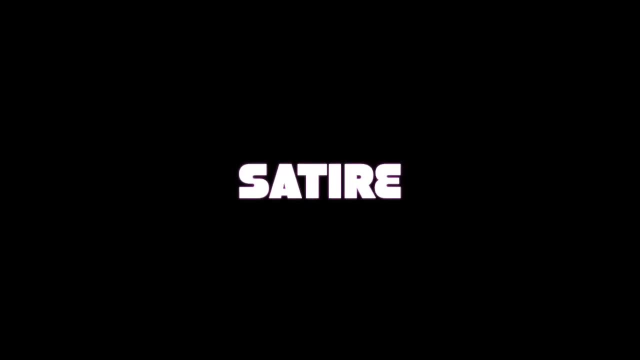 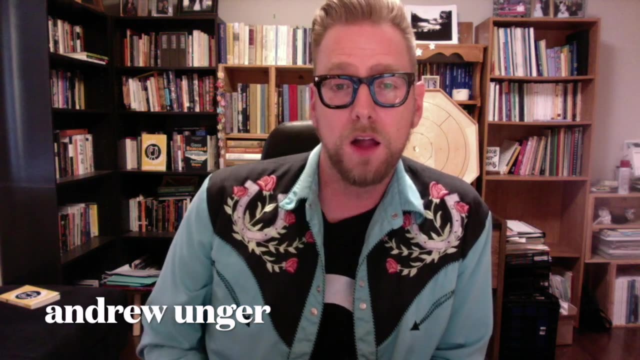 And that's what we're going to be talking about in this video. I'm Andrew Unger, author of the Mennonite satire website, The Daily Bonnet, along with my recent collection of satirical articles called The Best of the Bonnet, as well as 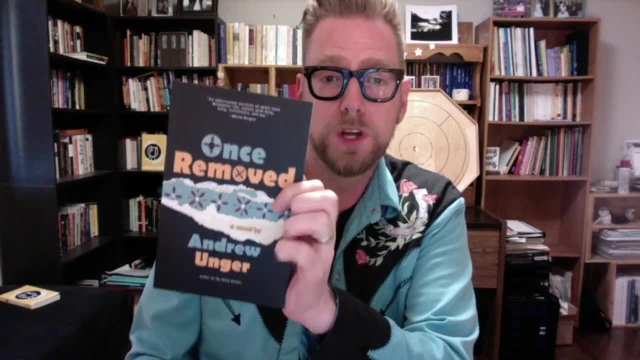 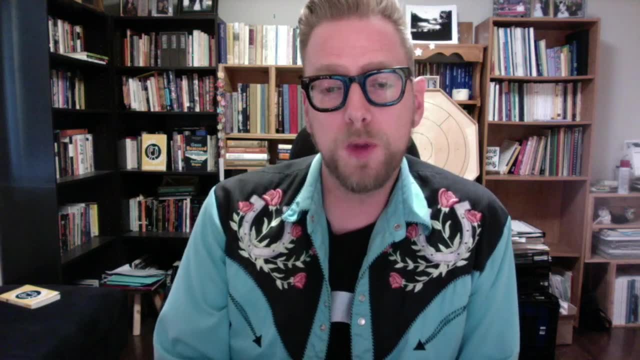 my novel, a satirical novel, called Once Removed. I'm going to run down the top five concepts that I think are most important to understanding satire. All right, so before we get into the top five, I think we should just start with a definition. 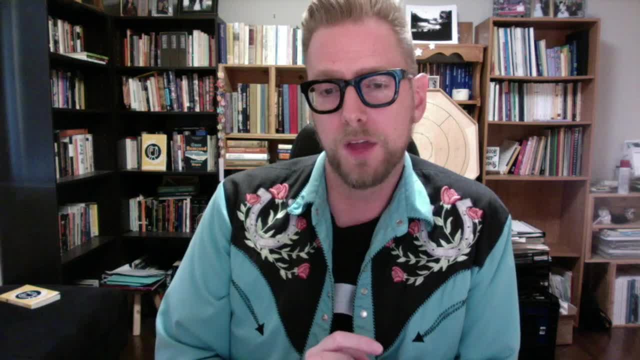 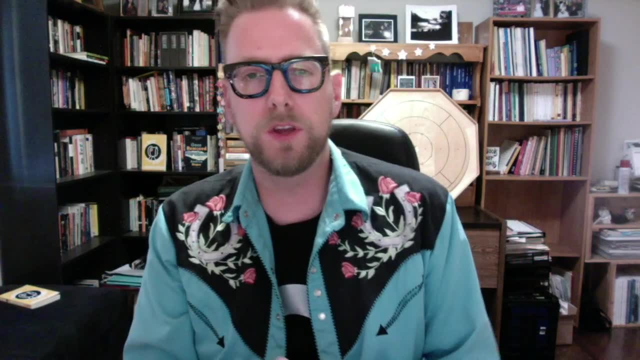 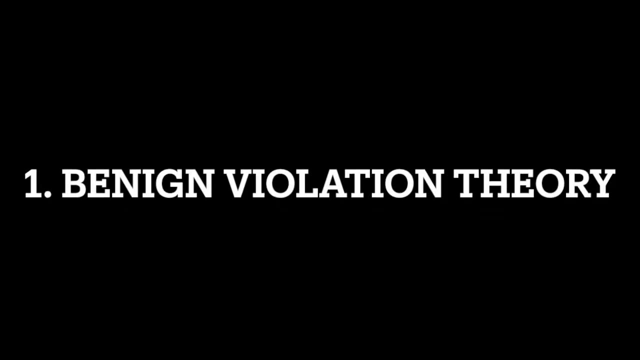 What exactly is satire? So satire is the use of irony, exaggeration and sarcasm to point out flaws in society. I'm going to come back to this definition when we talk about the difference between satire and parody, but I think for now that should be enough to get us started. 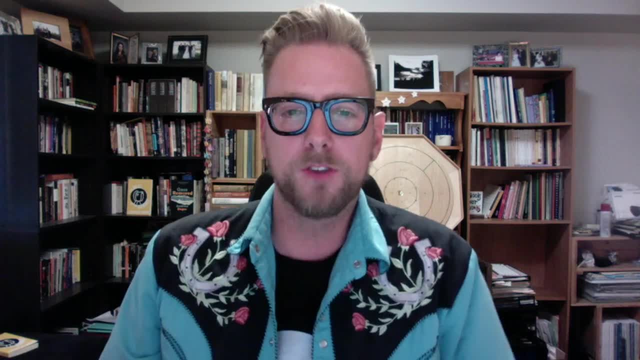 Satire is a form of comedy, or at least it can be, And so it's important to understand why do people laugh or why do people find things funny. A number of years ago, a scholar said: I'm going to tell you a story. I'm going to tell. 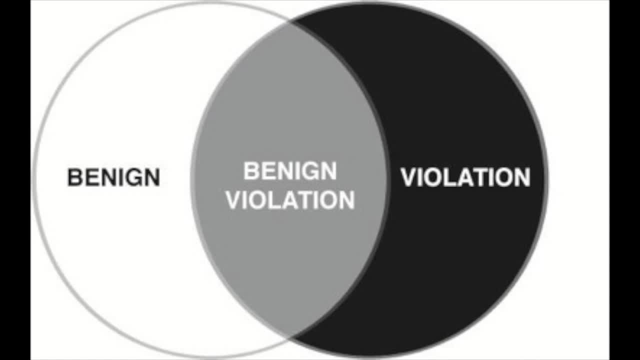 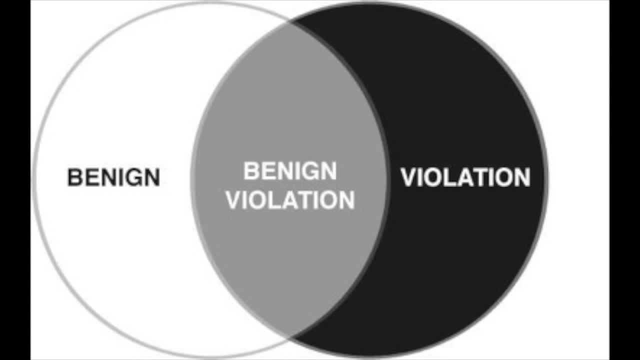 that people will find humor in situations that fall somewhere between being benign, in other words harmless, and a violation, in other words breaking a rule or social norm or an expectation, When these two factors are noticed simultaneously, and this is unconscious, of course, but when they come together simultaneously we laugh. We find humor in it When either 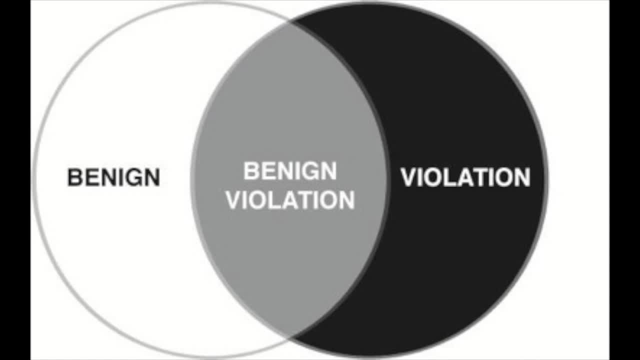 one is absent, we don't. We're likely at the bottom, But when one is absent, we can. We can don't. In other words, there must be some violation of social norms, rules or some kind of harm done. 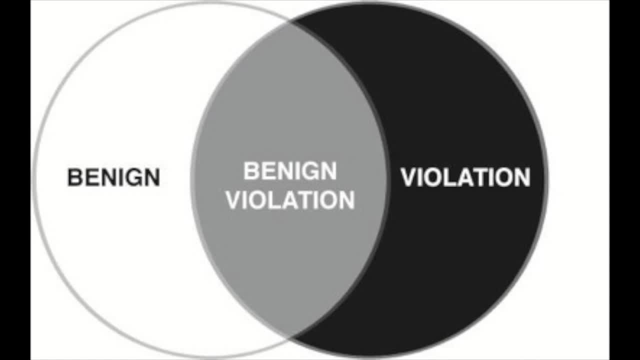 but it must be seen by the viewers as more or less harmless. You might laugh once you see someone else trip or fall, but not once you notice that they're severely hurt. In other words, it's a violation that they fell, but it's benign because they're not severely hurt, whereas if they're. 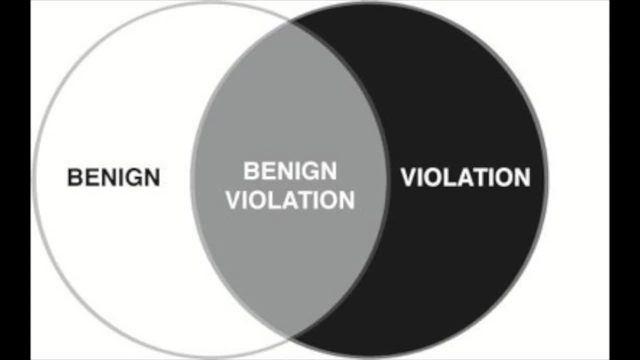 severely hurt. now, all of a sudden, that falls into the category of violation and it's not in that gray area anymore and you stop laughing- At least probably most people would. Another example that McGraw uses is tickling. Tickling, of course, is a violation of what. It's a violation of personal 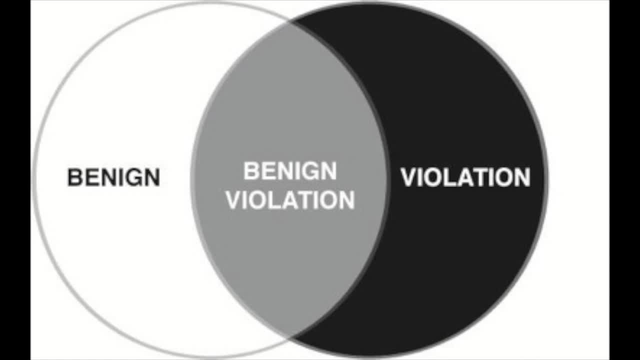 space. However, when you're tickled by someone you know and trust, you react by laughing because it's a benign violation. It's a violation, but it's benign. When you try to tickle yourself, however, you don't react at all because there's no violation, It's completely benign. On the other, 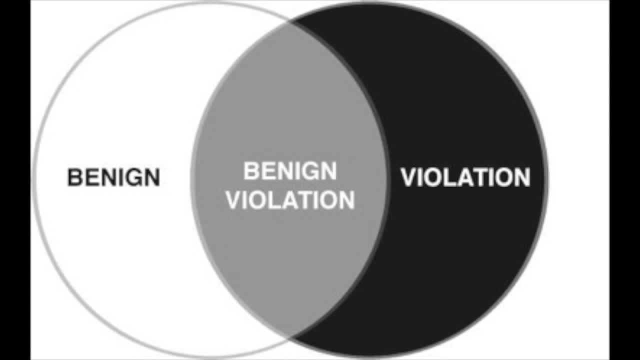 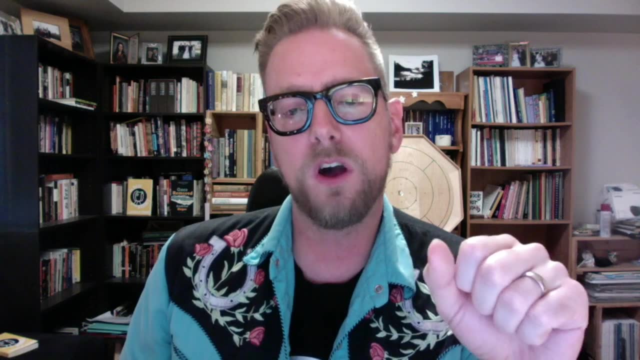 hand, if you attempt to tickle a random stranger on the street, the action will not likely be greeted with laughter and it'll be viewed solely as a violation and not benign at all. There's a great TED talk about this, which I'll link in the 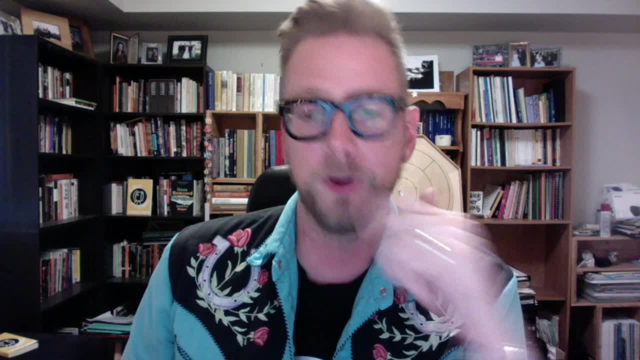 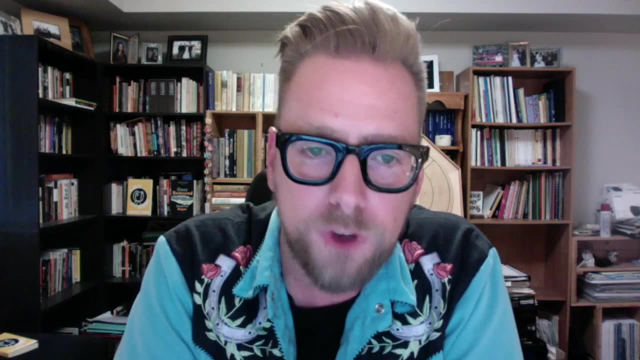 description below, where Peter McGraw explains this theory in much more detail for himself. I see this theory in action all the time on the Daily Bonnet. Whether someone gets the joke depends on them seeing the violation that's taking place. On the other hand, when someone takes 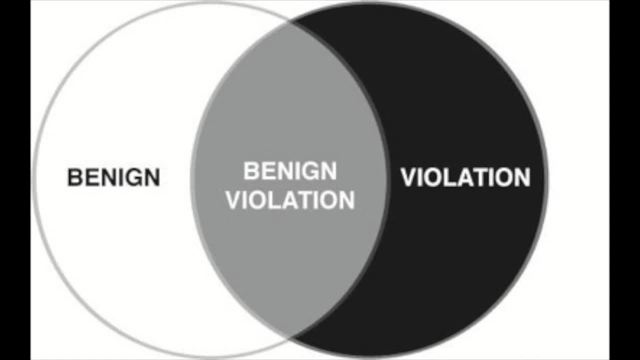 offense, it's because they don't see the violation as benign. They perceive that some sort of harm has actually occurred. The thing is, of course, that that gray area in the middle is different for each person, So what one person finds to be a benign violation, another person might find it. 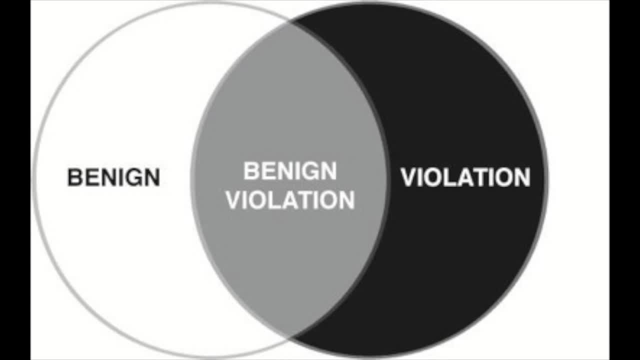 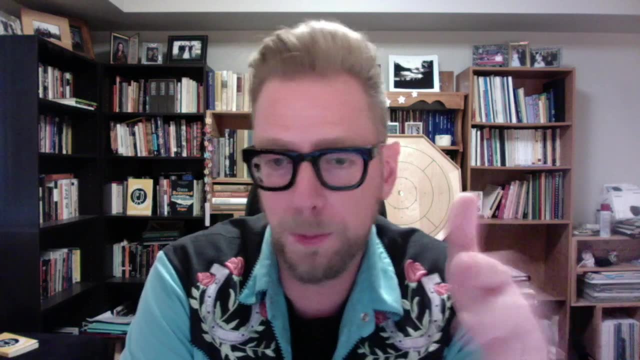 too benign to be funny and another person might find too much of a violation to be funny. You can apply this lens to almost any situation where people laugh or don't laugh, or some people laugh and other people don't laugh, and it works really well to explain why they did or didn't find it. 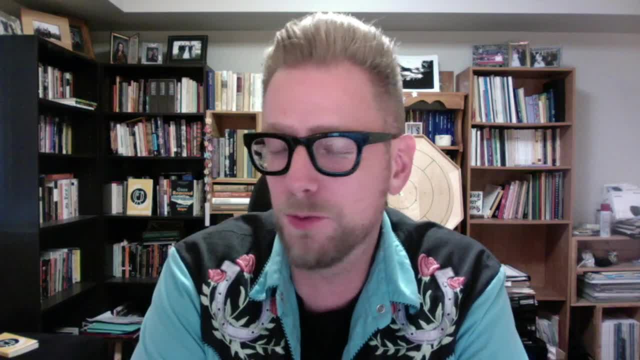 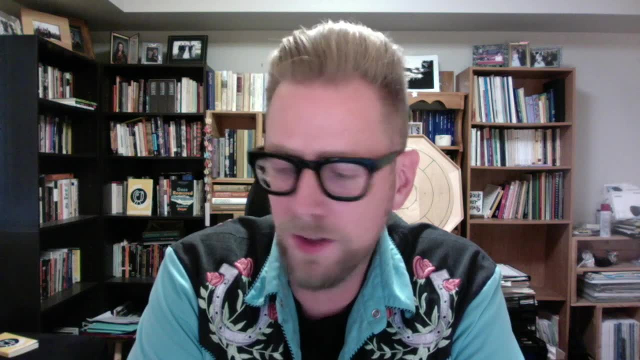 funny. This concept has also helped me to not really take it too personally when, on rare occasions, people have been upset with things that I've written because I just go. well, you know, I guess it was in the violation area for them, but for other people it was a benign violation. 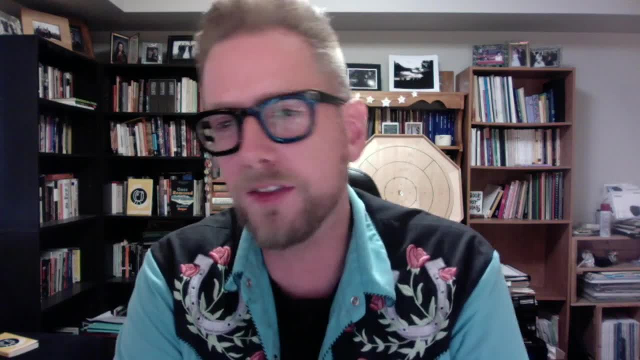 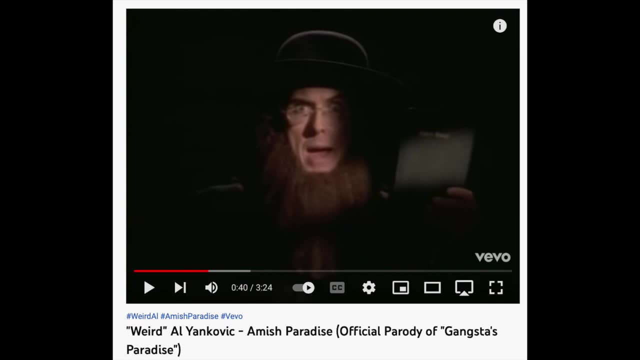 A concept number two, and that is the difference between satire and parody. On the surface, satire and parody have a lot in common. When you look at a Weird Al Yankovic video where he parodies popular songs, you see that it has a lot of things in common with satire. 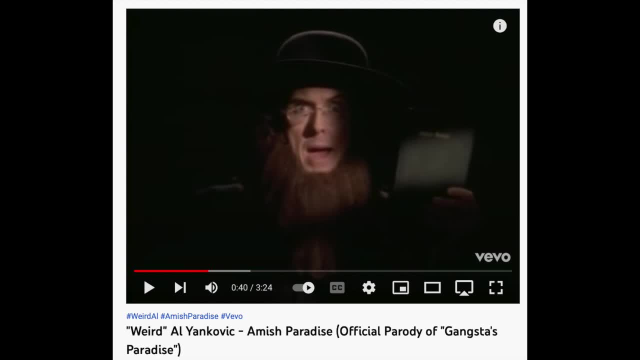 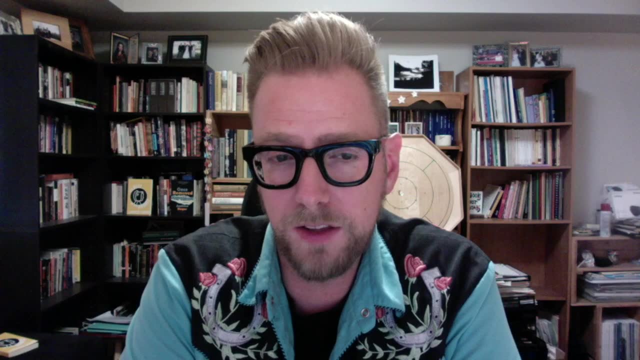 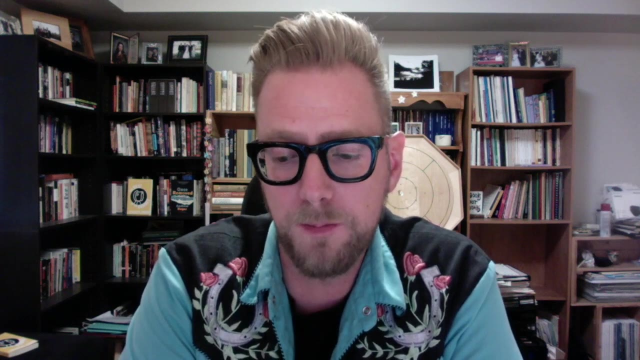 It uses imitation, it uses exaggeration, it has humor, and so on. However, the big difference between the two is that satire is intending to make some sort of a point by pointing out a flaw, whereas parody is simply. the humor simply comes from recognition of something being similar. 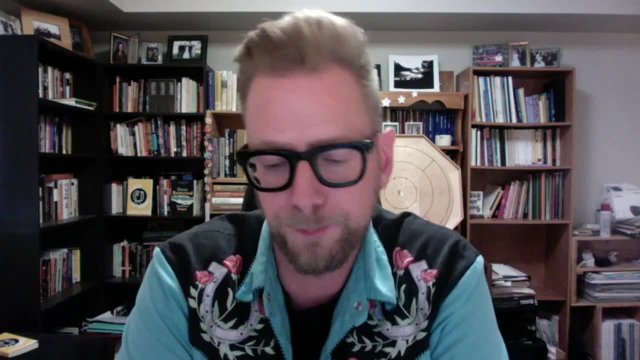 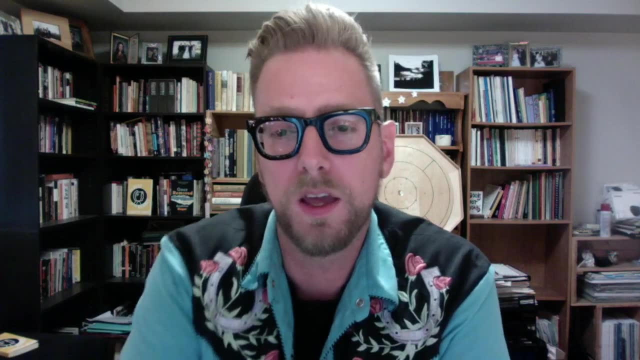 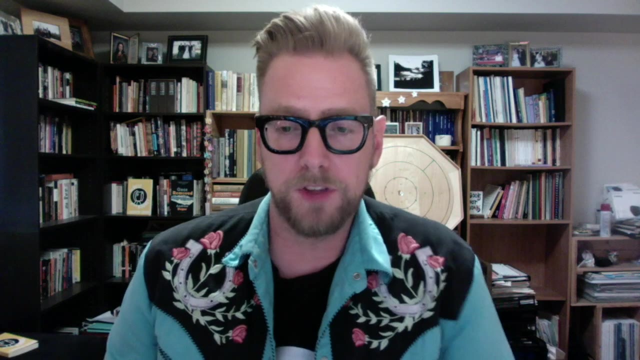 or you're taking something and you're just twisting it. Although a lot of people describe the Daily Bonnet as a satire website, a lot of the articles on the website are actually- would be more accurately described as- parody, So let me give you a couple examples here. 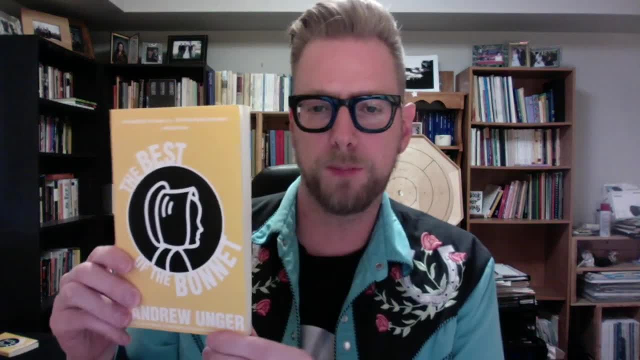 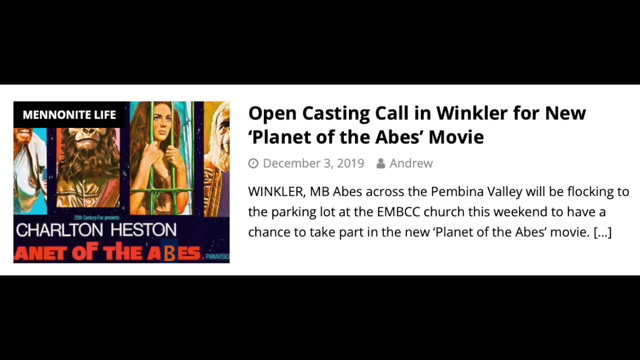 So both of these examples are actually in The Best of the Bonnet, so you can find them there if you're interested. So the first one let's look at is with the headline: Open Casting Call on Wink. Now, if you aren't unfamiliar, the name Abe, which would be short for Abraham, is a common. 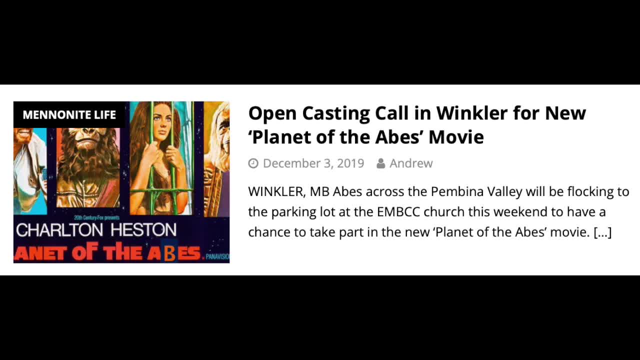 Mennonite name and Winkler is a town with a lot of Mennonites and therefore it would have a lot of Abes. So the joke here is really just a pun, a play on words, and then of course, it's a parody. 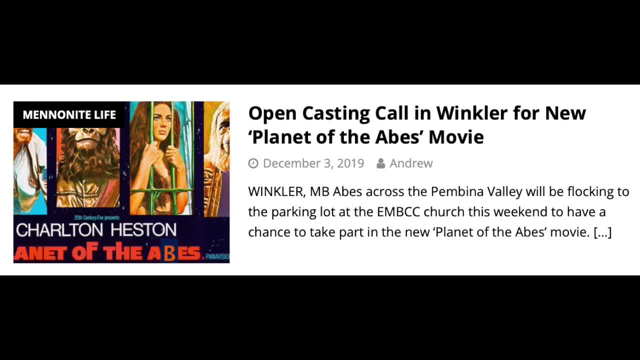 on the movie Planet of the Apes. Rather than Planet of the Apes, we have Planet of the Apes and of course they're going to cast characters, cast actors in Winkler, because there's such a high number of Abes, Abes with a B in the area. 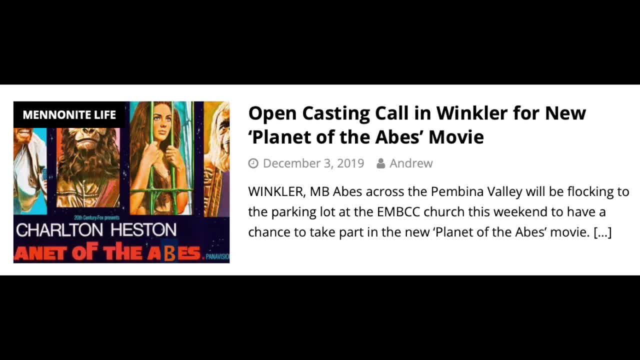 This is simply parody. This is not satire because it's not making any kind of a point. It's not like I've got some subtle critique on people named Abe or on Hollywood movie industry or anything like that. This is a parody, Of course. the other way in which the Daily Bonnet 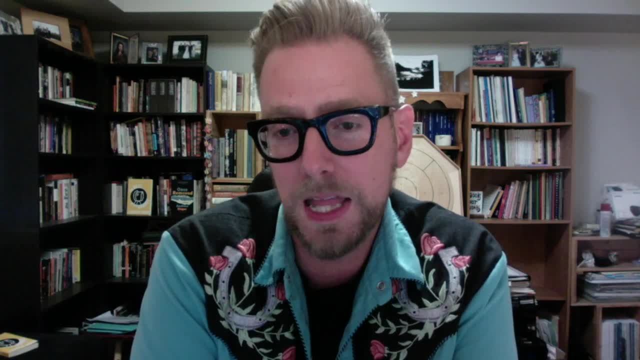 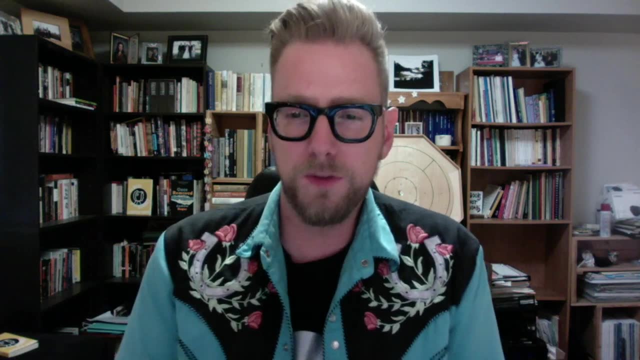 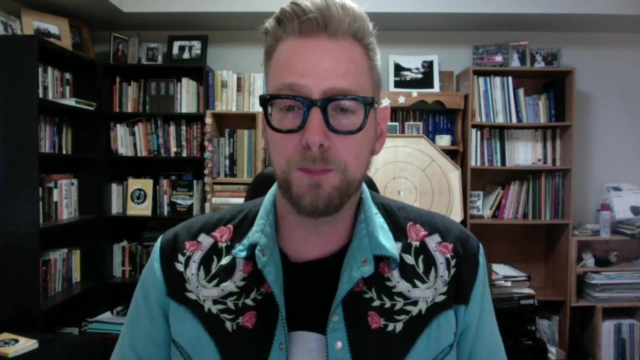 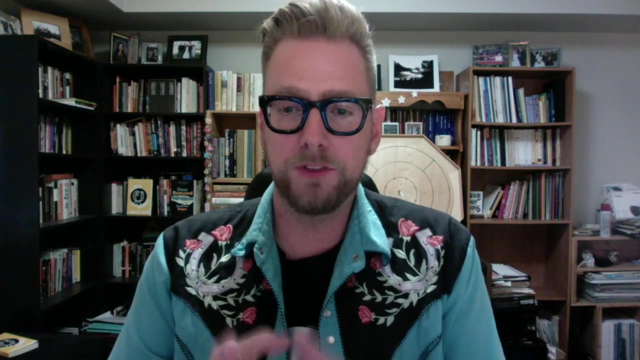 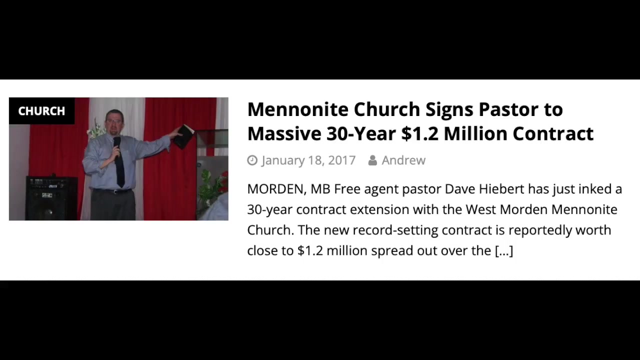 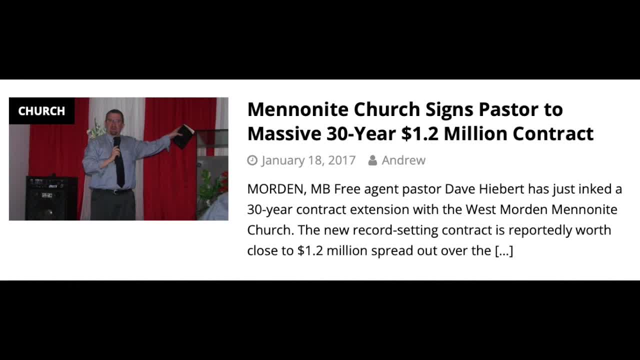 a year $1.2 million. contract readers will immediately see, if they do the math, that $1.2 million spread out over 30 years is not a heck of a lot of money by North American standards, and therefore the point of this article is immediately clear that it's a critique. 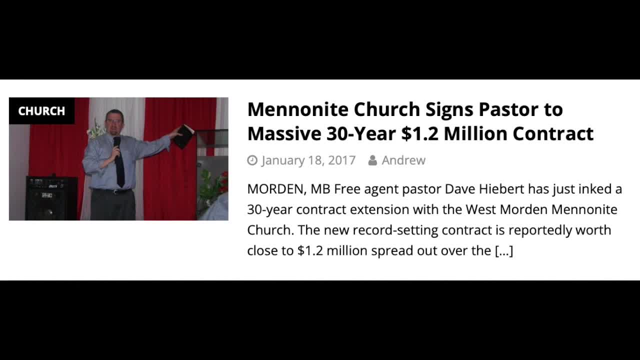 on how little Mennonite pastors get paid, especially in comparison to people like professional athletes. So you could say that this article has two points, one being a critique on how low pastors get paid and second being a critique on how much money is spent on professional 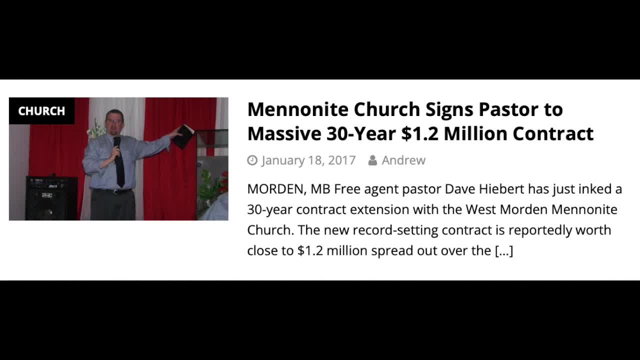 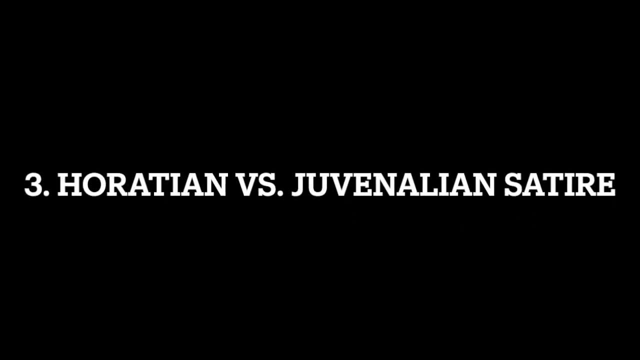 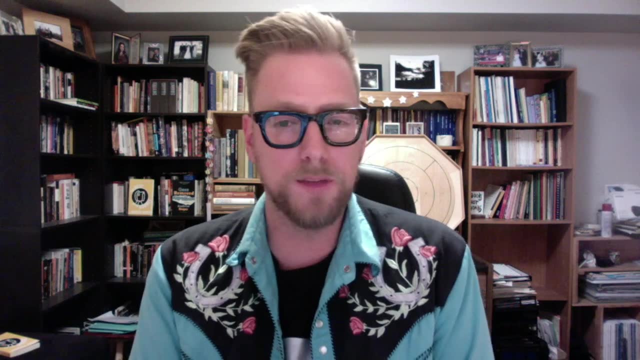 athletes. It's kind of making both of those points. This, of course, is an example of satire, because it uses exaggeration to make a point. All right point, or concept number three, And that is understanding the difference between Horatian and Juvenalian satire. 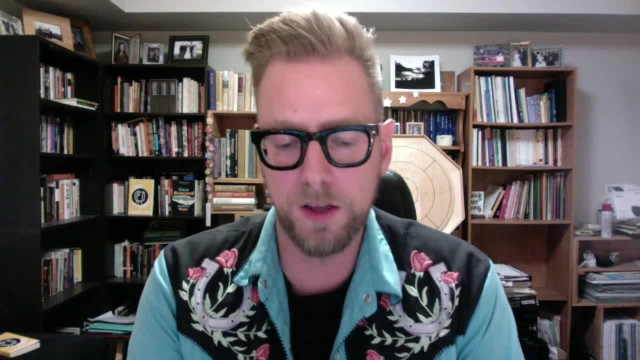 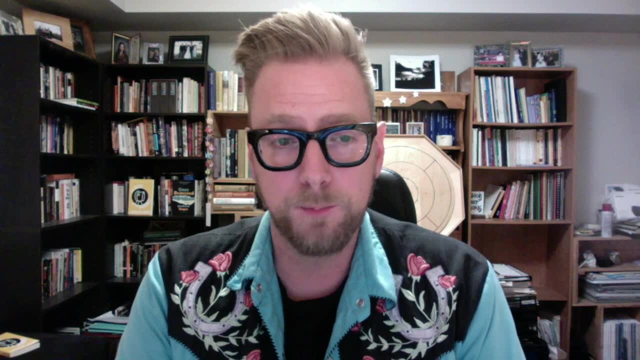 Now, a lot of people know that there's, of course, different types of satire in terms of the form that's being used. So, for example, you have news style satire, and then, of course, you have satire being used in movies and stand-up comedy and other forms of comedy as well too. 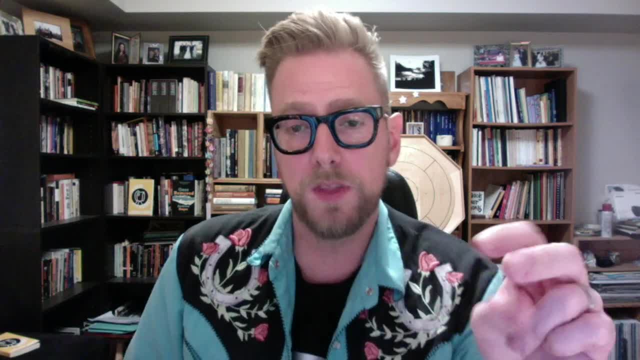 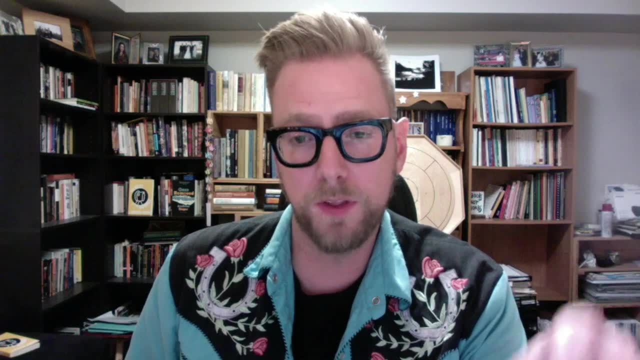 But that's not really what we're talking about here. The difference between these two forms of satire has nothing to do with the form that's being used. It's the form that's being used That has everything to do with the tone that's being used. I can remember when I was a kid. 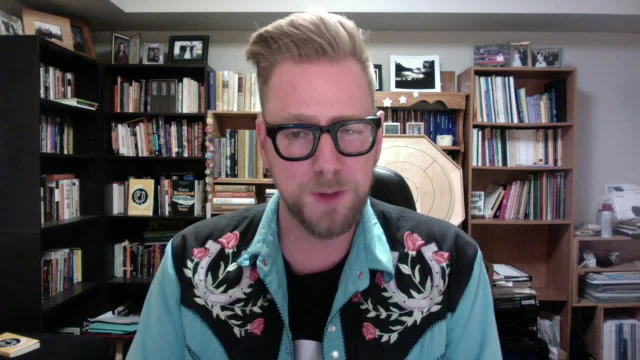 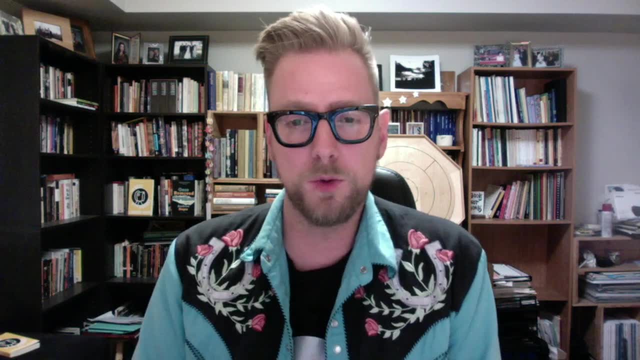 didn't happen too often, but occasionally my mom would say: don't speak to me with that tone. And that's what we're talking about here, The tone that's being used in the writing, And a little bit has to do with the message. I'm not going to get too much into the origin. 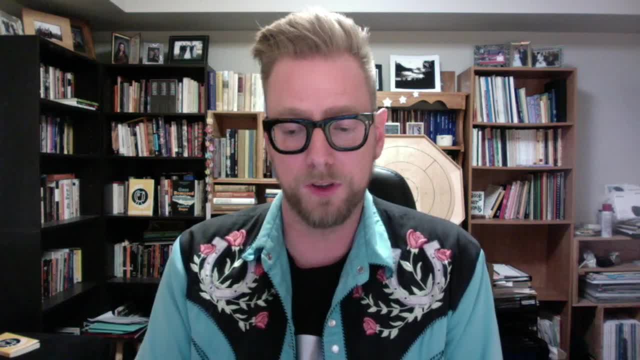 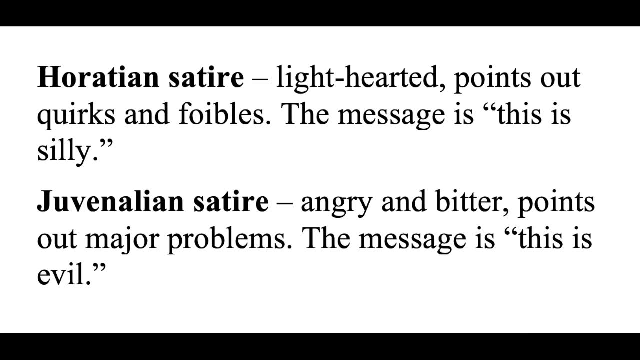 of these names but they come from ancient Roman satirists. And the Horatian satire is the more lighthearted satire. It's the kind of goofy, lighthearted, fun, funny satire. The second type is the Juvenalian satire, which is harsh and bitter and angry. 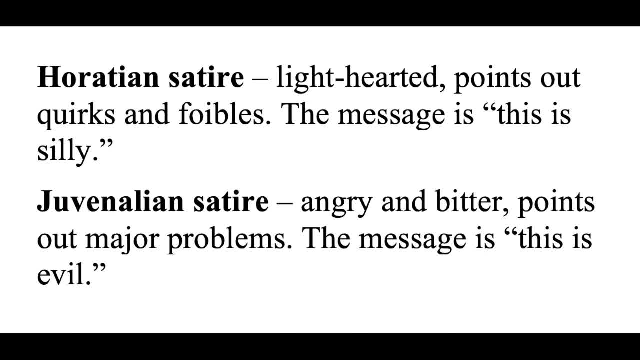 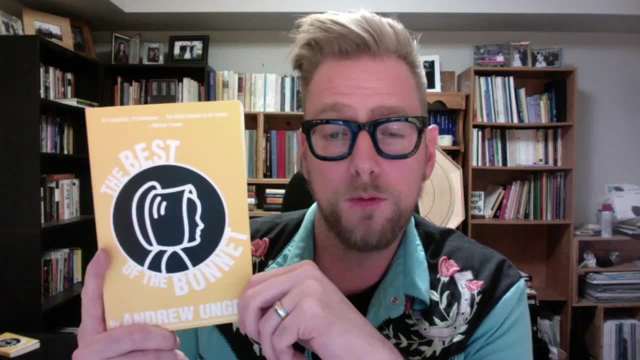 So the message I would say of Horatian satire is: this is silly. The message of Juvenalian satire, I would say, is: this is evil, And you could probably see right away how those both have uses. So I would say that the vast majority of the articles in the Daily Bonnet would fall into 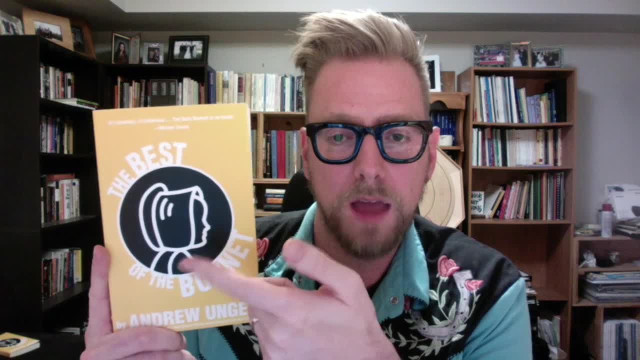 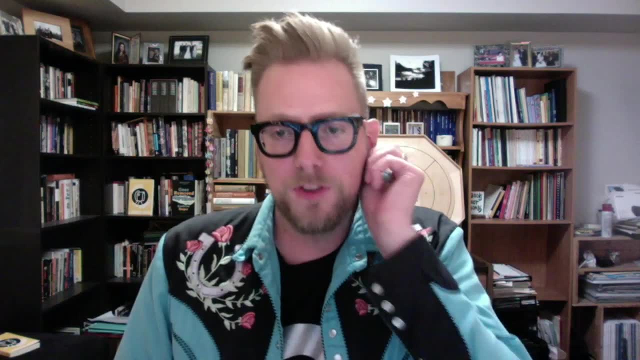 the category of Horatian satire. And in fact there's an essay in the back of the Daily Bonnet- the best of the Bonnet- where scholar Nathan Dweck makes the case that the Daily Bonnet is in fact Horatian satire. Here's an example of Horatian satire for you. 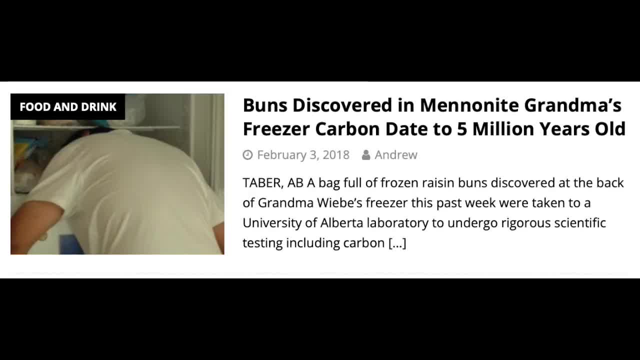 Buns discovered in Mennonite grandma's freezer carbon date to five million years old. I'm sure you all can relate to going over to grandma's house, looking in the freezer and wondering exactly how long those frozen items have been in there. Now this is exaggerated, of course. 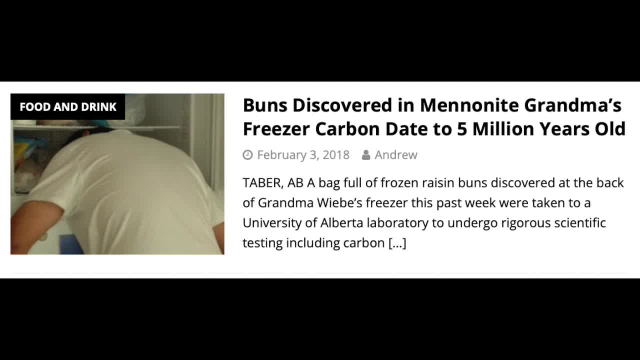 which is what makes it satire. But this is Horatian satire because although it's a critique of grandma, in a way it's a very light-hearted critique. It's not angry at grandma, It's just saying, hey, grandma, like you got some buns in your freezer that are a little old, you know. 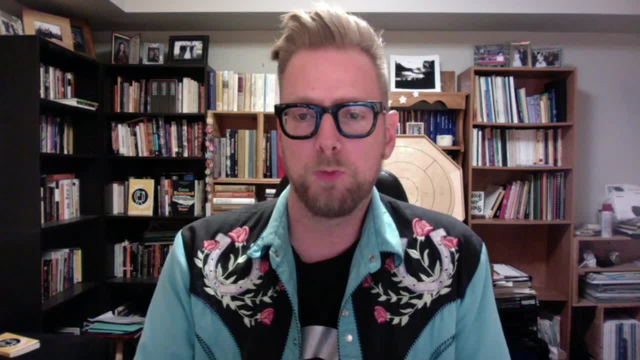 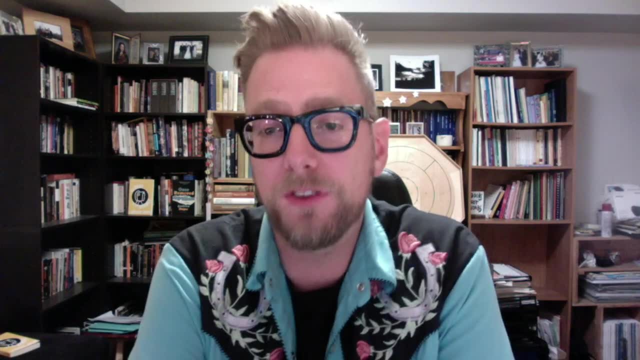 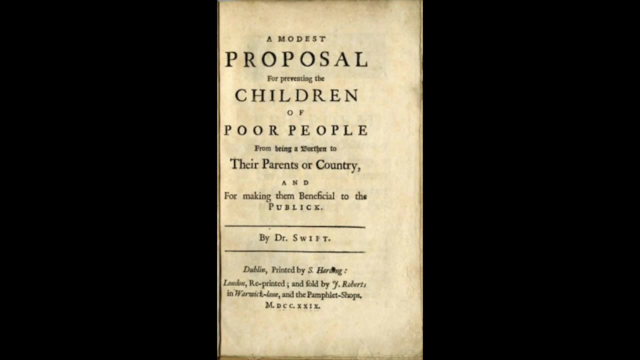 It's very light-hearted. It's saying this is a quirk at worst. It's not angry. It's not saying this is evil. A very famous example of juvenilean satire is the example that I started this video with, and that is Jonathan Swift's Modest Proposal When you're dealing with major social issues. 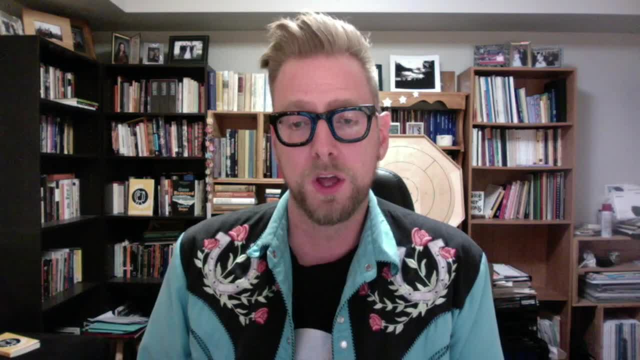 sometimes you're dealing with a lot of things that are not social. And when you're dealing with a lot of things that are not social, sometimes you do have to be angry and you have to have that kind of tone. He was addressing the problem of poverty in his society and he couldn't just sort of 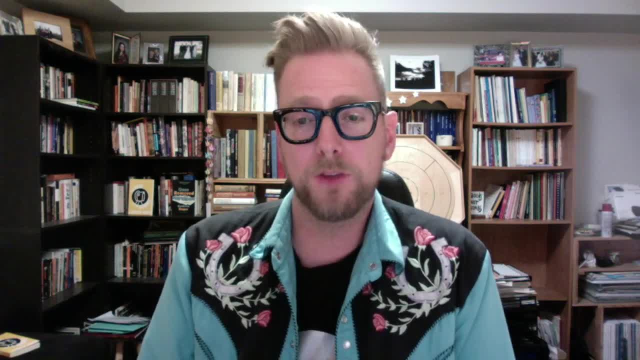 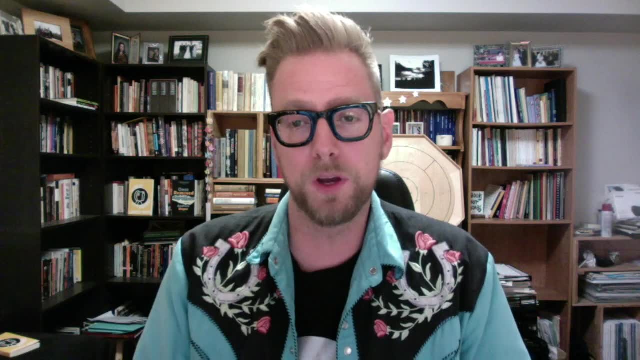 joke it off or do a sort of light-hearted thing with it. That is why, if you read it, it does come across funny, but it also has definitely a sort of a bitter angriness to it, which is the key characteristic of juvenilean satire. 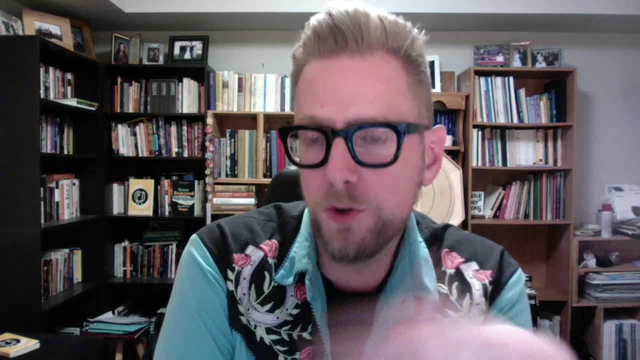 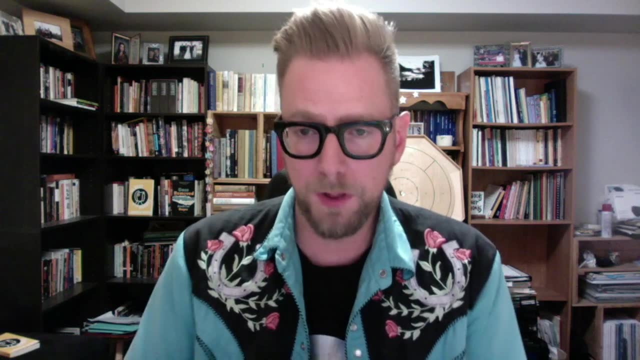 All right. concept number four, And that is the two main types of exaggeration. Usually, when we think of the word exaggeration, we think of what is actually called hyperbole. That is where people are overstating something. Satirists will stretch things for humorous effect. So the examples that I've given you so far have 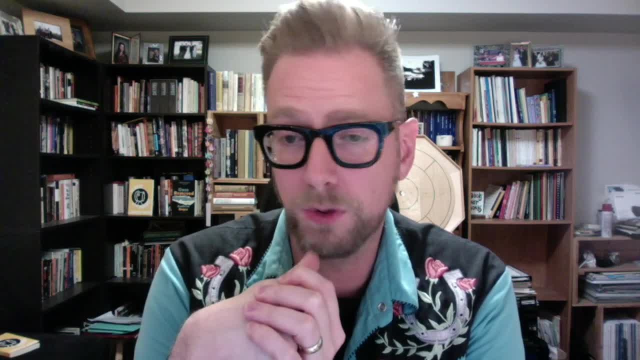 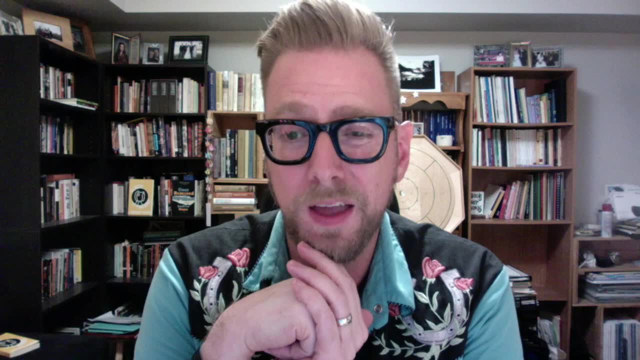 all been examples of hyperbole: The buns that were a million years old, or the pastor who signed this really huge contract, or even Jonathan Swift's Modest Proposal where he's proposing cannibalism. It's more extreme and too extreme to be real. 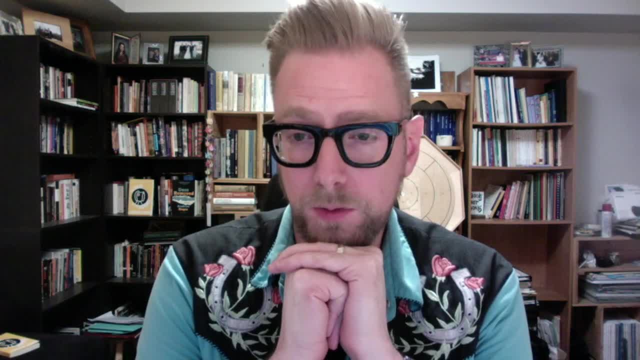 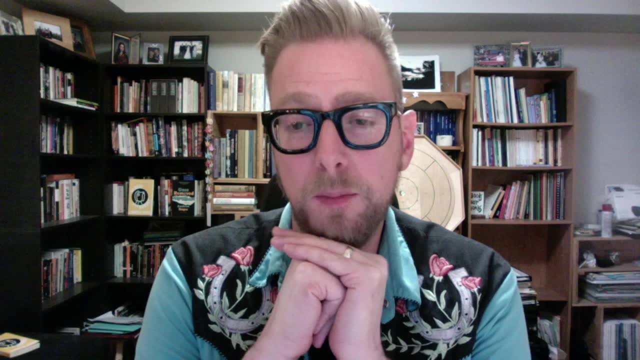 So those are all examples of hyperbole, or what we would what, in casual speak, we would just call exaggeration. There's actually another kind of exaggeration, and it's commonly used in satire, although not as much in the headlines. You can find it within articles if you look for it, and 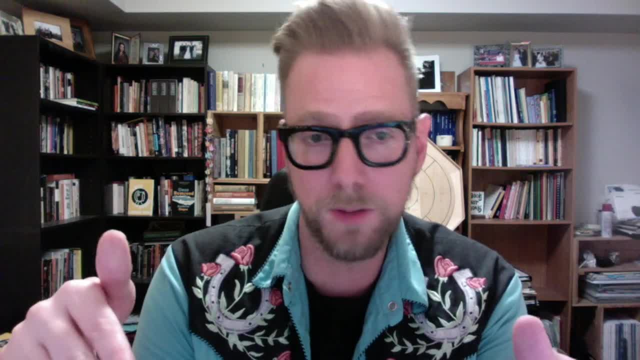 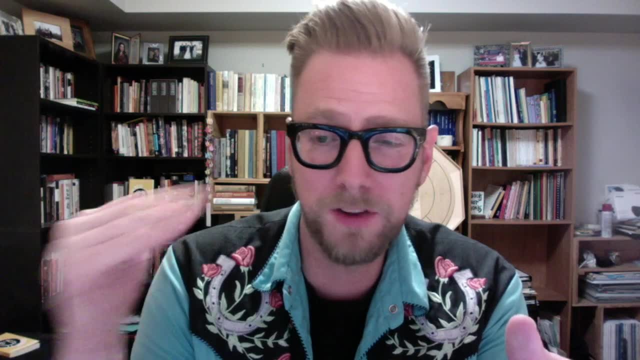 that is understatement, where you're sort of downplaying something. Instead of saying it's more than it is, you're saying it's less than it is, And there's humor there. It's maybe a little more subtle, but it sometimes can be used very effectively. 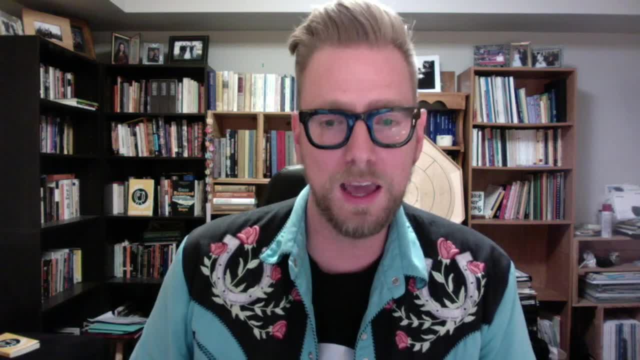 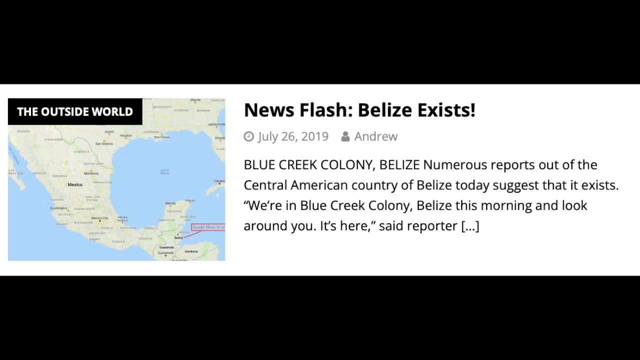 So one example of where I did use it in a headline is this one where it says: Newsflash- Belize exists Now. Belize is a very small country in Central America where there's a significant Mennonite population, which is why I wrote an article about it. But basically, instead of saying that anything 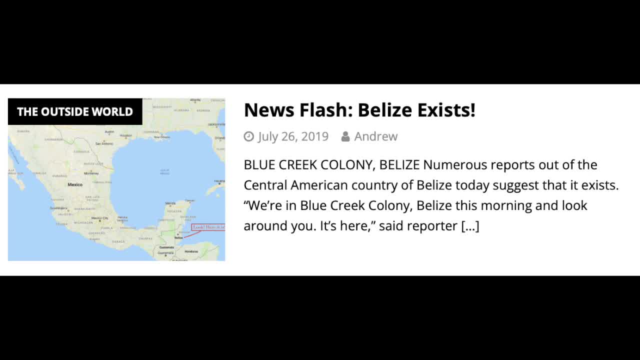 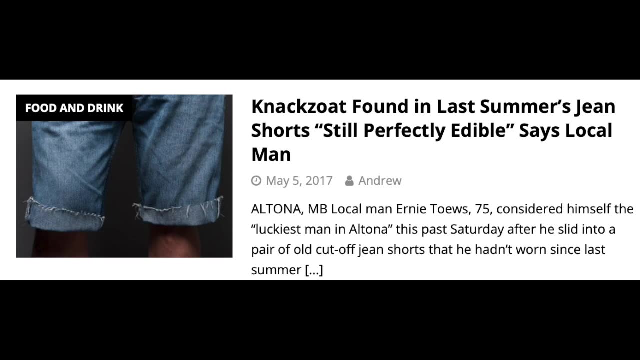 happened there. the idea was that people aren't even aware of its existence, And so I'm simply just saying: Belize exists. Another way that news-style satire commonly uses understatement is to take everyday occurrences and report on them as if they're newsworthy. This would really be an 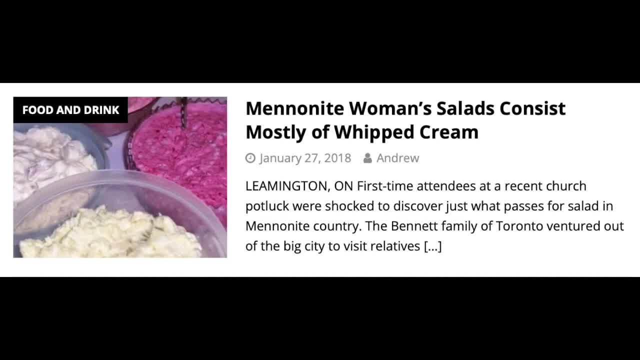 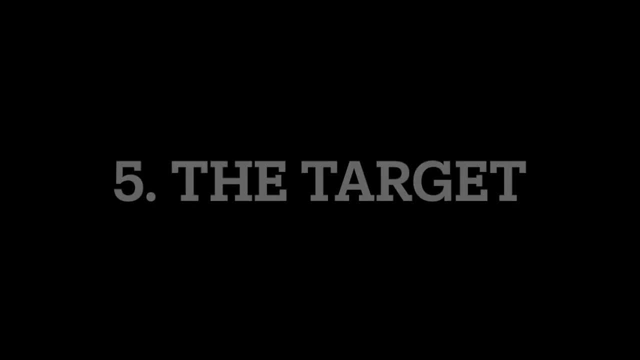 example of observational humor, where the joke comes in simply going: oh yeah, I do that too. Concept number five: the last concept that I think is important to understand when understanding satire, and that is: who is the most important person in the world And that is who is the most. 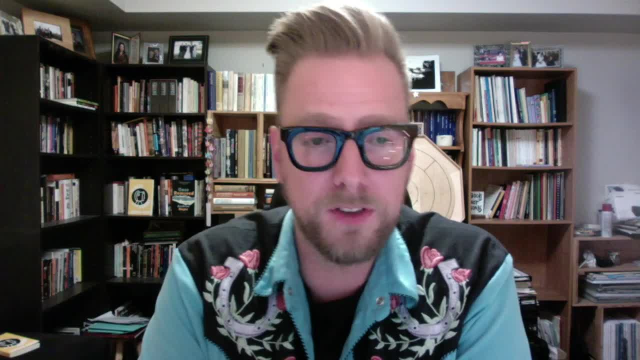 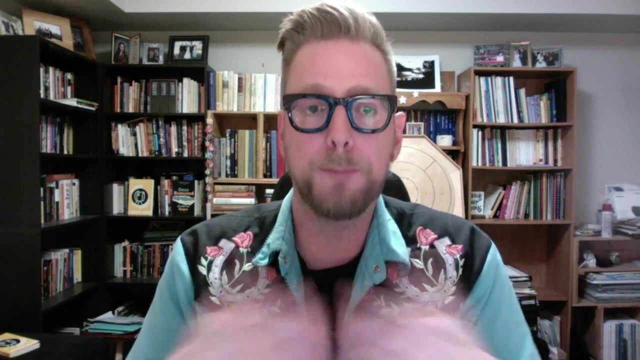 important person in the world, And that is who is your target. Whether you're reading satire or writing satire, it's important to think about who your target is. Now, of course, the target, that is, the person or people or personality trait that's being made fun of in the satire- can really run. 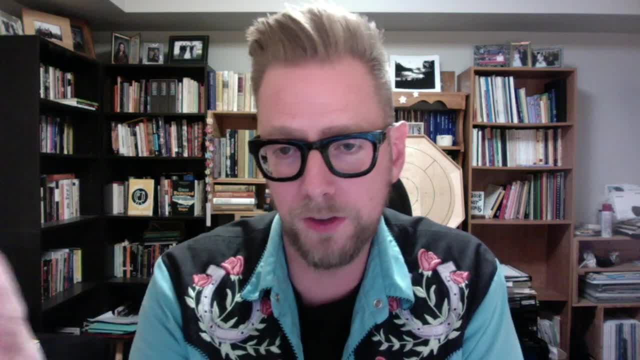 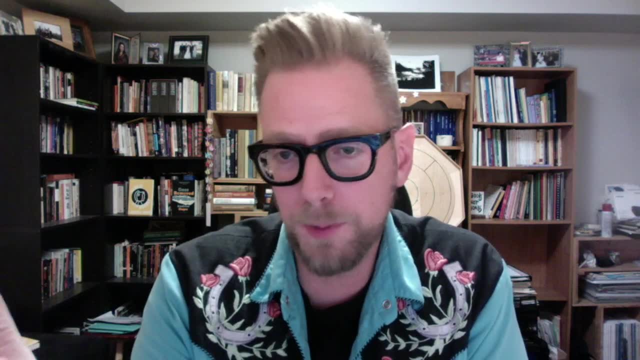 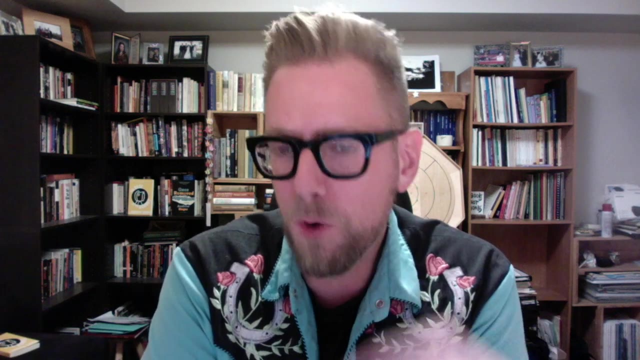 the spectrum from everyday people to celebrities, to even just general personality types. as I said, Sometimes you're referring to very specific, identifiable people and sometimes you're referring to more general people that tend to do certain things right. But I think, even more important than being 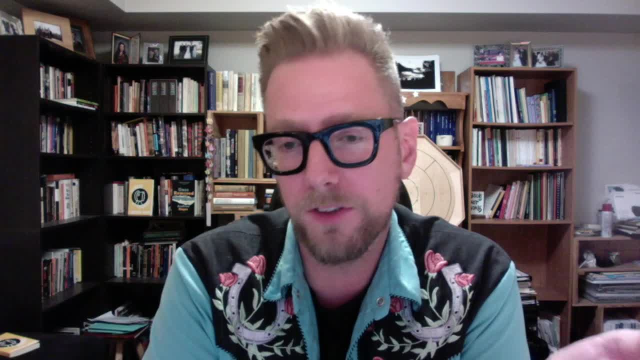 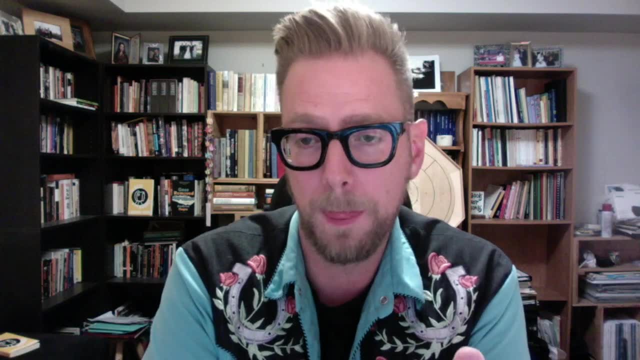 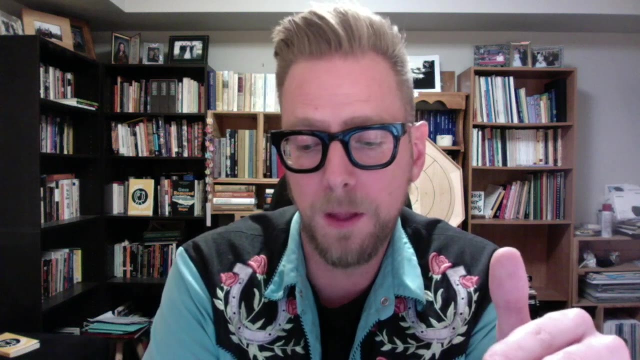 able to correctly identify the point or understand the message or target of the satire is to look at the question: is the satire punching up or punching down? This, of course, is a metaphor from boxing or something like that. When you punch up with satire or with comedy in general, you are using 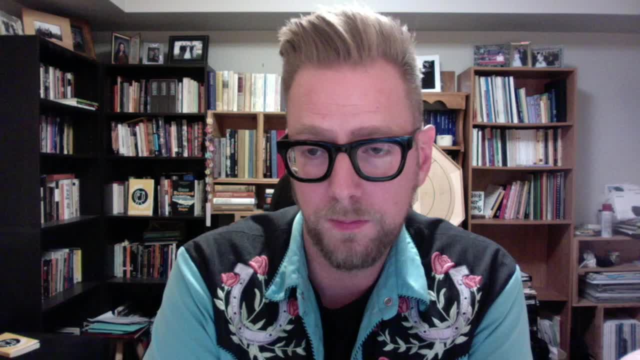 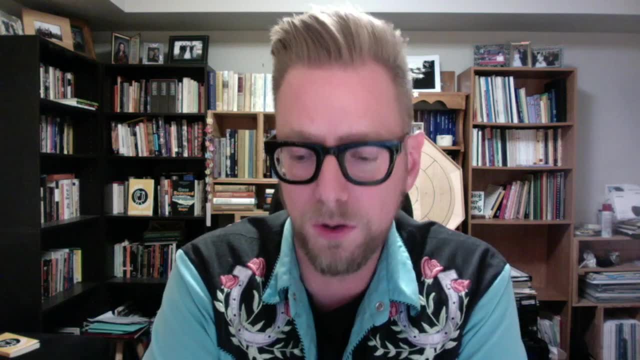 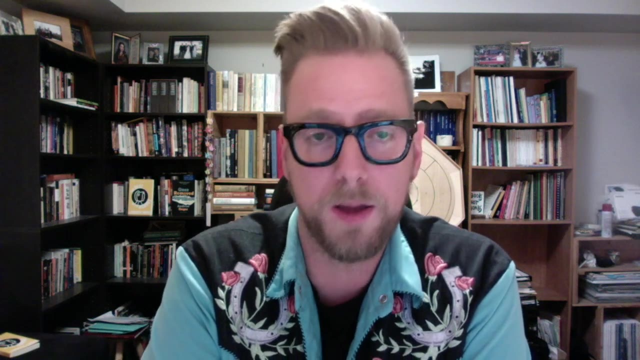 your satire to critique the powerful people in society, And that is what the goal is. Satire, from the ancient Romans to Jonathan Swift through to today, really is intended to do. When you're using satire to punch down, you're now using it to make fun of or mock marginalized people. Is it possible to write satire that does that? Yes, There are some satire websites, unfortunately, that spend a lot of time doing that. Instead of using satire to challenge a reader's perception of the world, they just use satire to confirm what the reader already thinks. 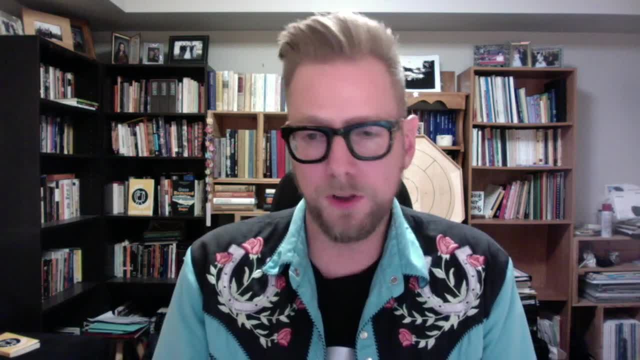 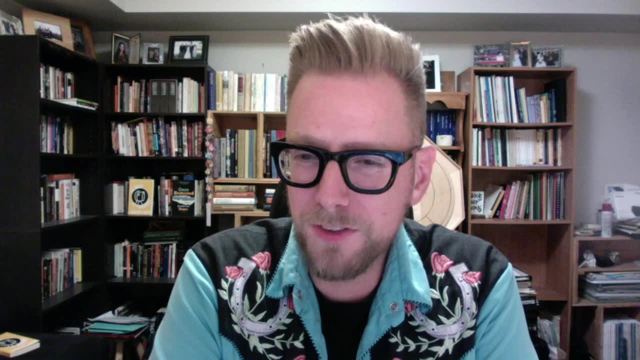 So these are some of the questions that I like to think about when looking at the target of satire, But it does raise questions for me. Is the Daily Bonnet punching up or punching down? Well, maybe it's neither. Maybe in this case it's punching inward or sideways, Because I am writing. 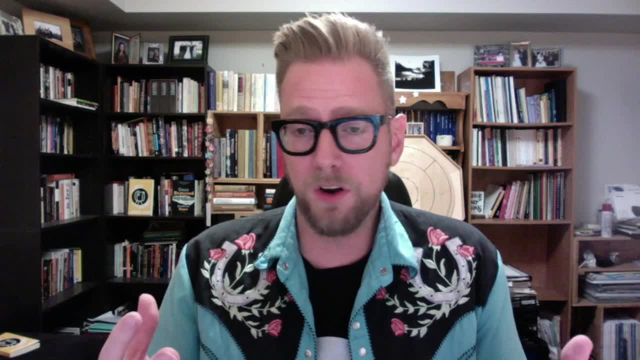 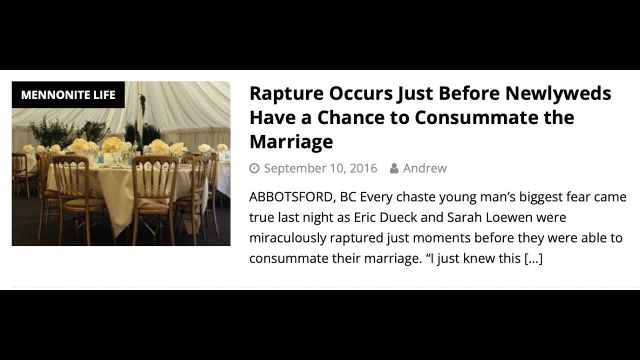 about my own cultural and religious background, and oftentimes the articles are very autobiographical. For example, this is a little embarrassing to say, but this article with the headline right here: Rapture Occurs Just Before Newlyweds Have a Chance to Consummate the Marriage is based on a real fear that I did have as a teenager. 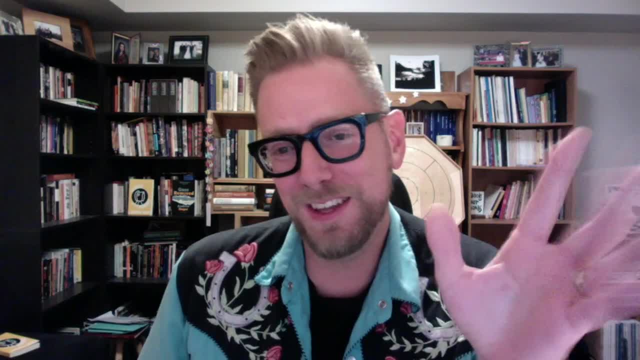 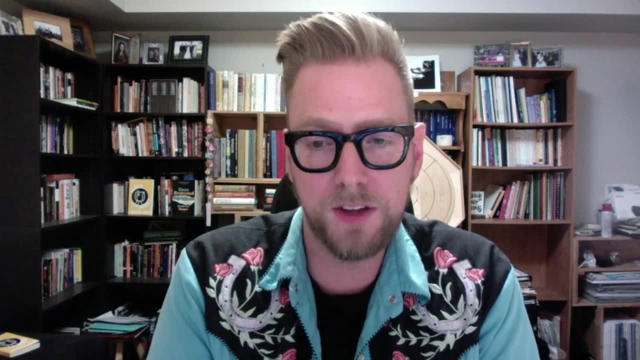 youthful Mennonite paranoia. Thankfully, it turned out fine for me. So those are my five concepts that I think are important for understanding satire. There's a lot more to it than that, but I think this is a good start If you're interested in more information.